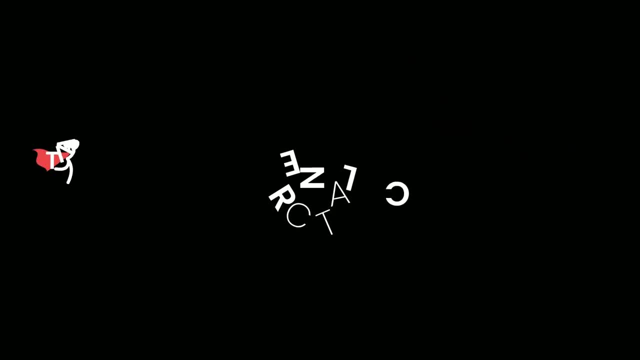 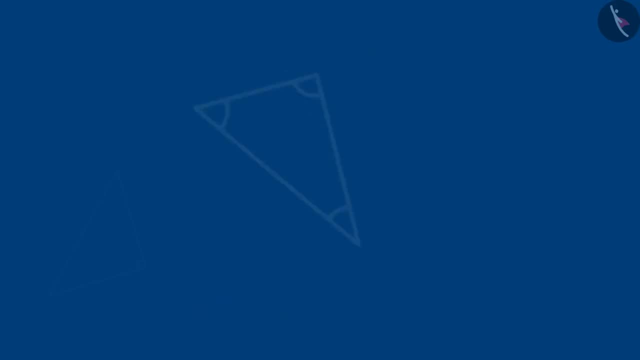 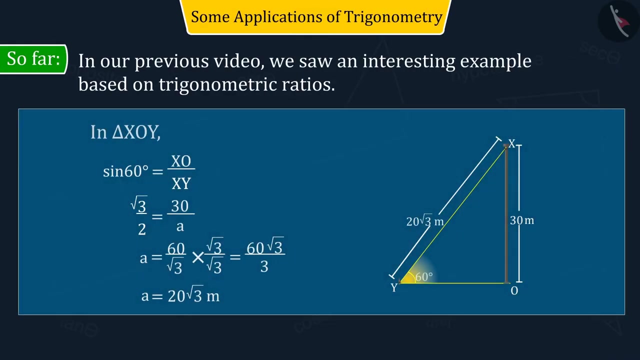 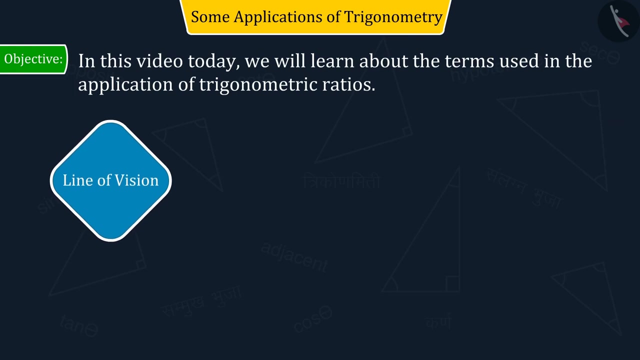 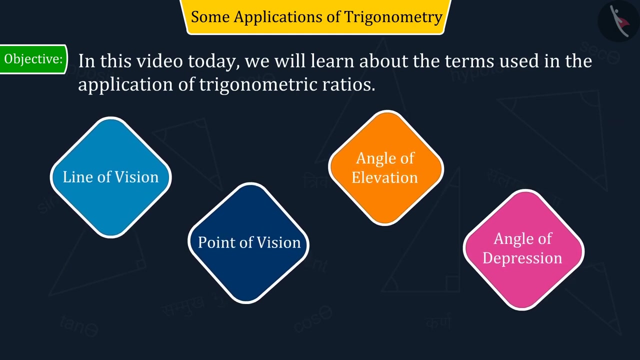 Welcome to this video. In our previous video, we saw an interesting example based on trigonometric ratios. In this video today, we will learn about the terms- line of sight, point of view, angle of elevation and angle of depression that are used with trigonometric ratios. 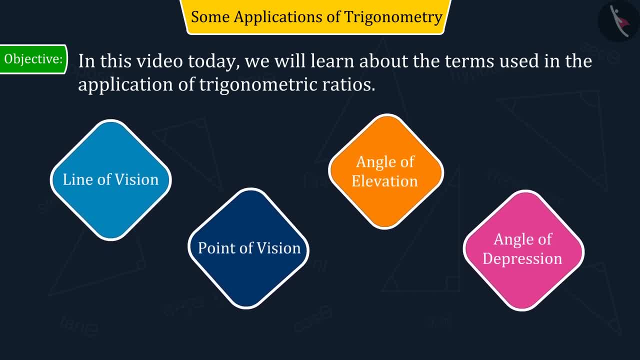 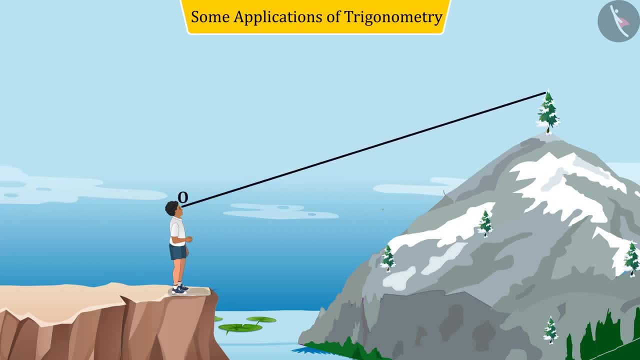 So let's discuss these terms. When a person sees the top point P of an object from his point of view, ie point O, the line OP joining these two points is called the line of sight. So we can say that the point from which the object P is seen is called the point of vision. 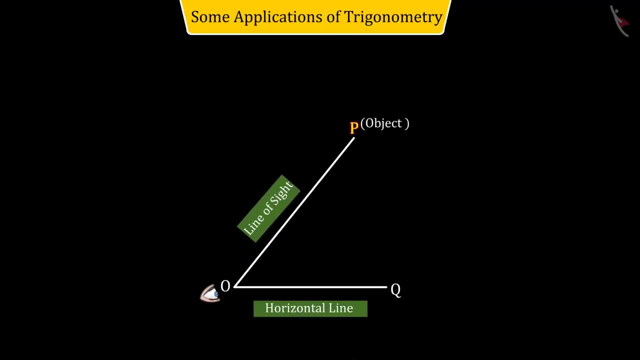 If an object P is above the person's eye, ie the horizontal line OQ passing through point O, then for the person to see that object, the angle by which he has to raise his vision relative to the horizontal line is called the angle of elevation. 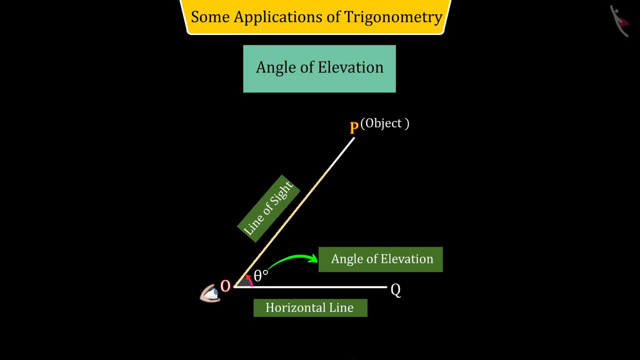 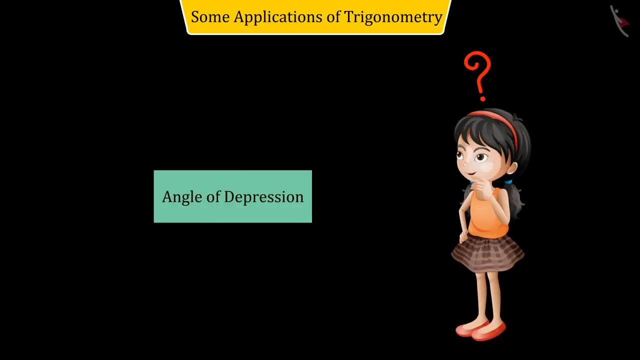 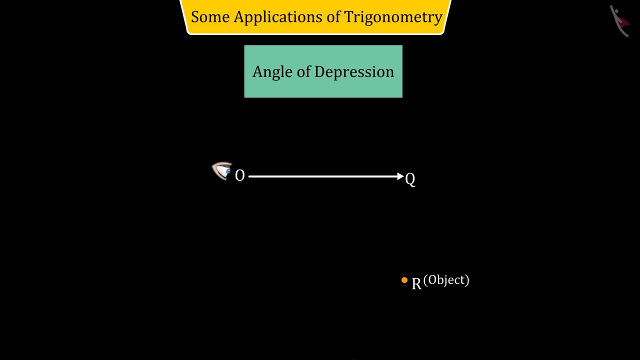 So with the help of an image we can tell that angle. POQ made from line of sight and horizontal line is called the angle of elevation. So now can you tell what is the angle of depression? Absolutely correct. If an object lies below the horizontal line passing through the person's eye, then 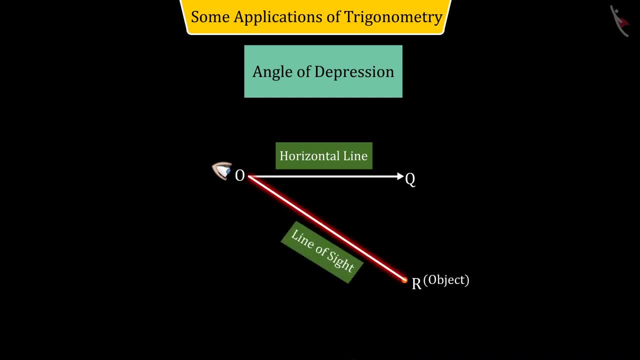 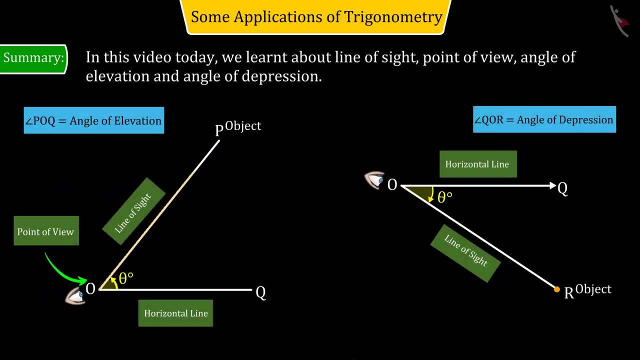 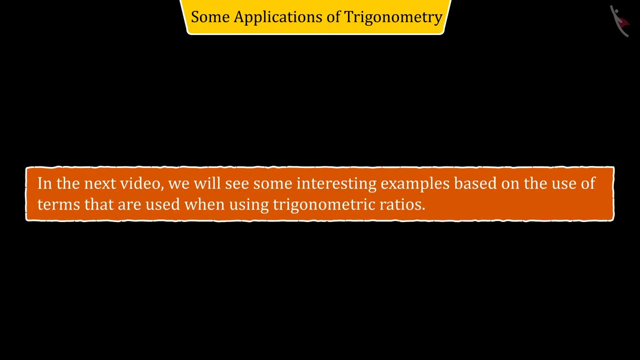 the angle QOR formed between the line of sight OR and the horizontal line. OQ is called the angle of depression. In this video today, we learnt about line of sight point of view, angle of elevation and angle of depression. In the next video we will see some interesting examples based on the use of terms that are used when using trigonometric ratios. Thank you for watching.